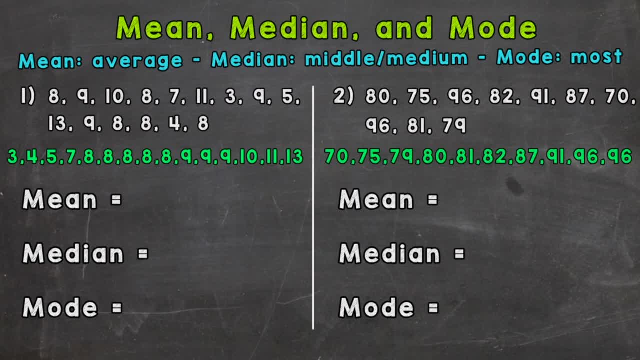 And, as you can see on your screen, we have number one to the left and number two to the right, So we're going to find the mean median and mode for each of those. So let's hop right in to number one. 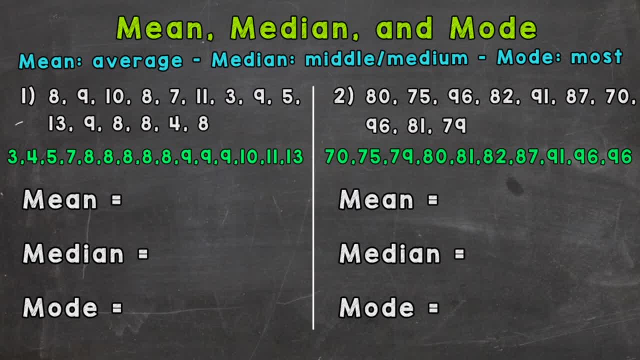 So for number one, we have a list of numbers up here. This is our data set Now below it in green: this list I already put in from least to greatest. So I put those numbers from least to greatest to help organize them. 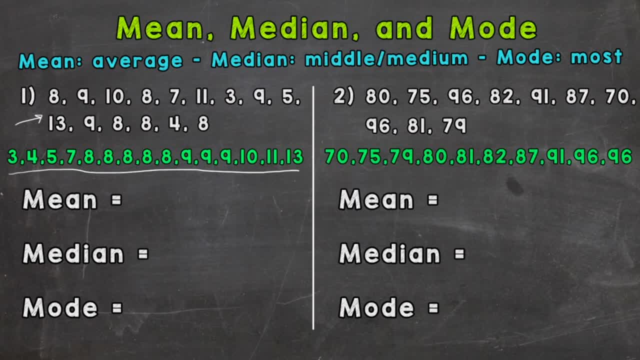 So whenever you have a list of numbers, order them from least to greatest first. Then we can find the mean, median and mode. So let's do mean first. And the mean is the typical average we think of when we add up all the numbers in the data set and then divide by how many numbers there are in that set. 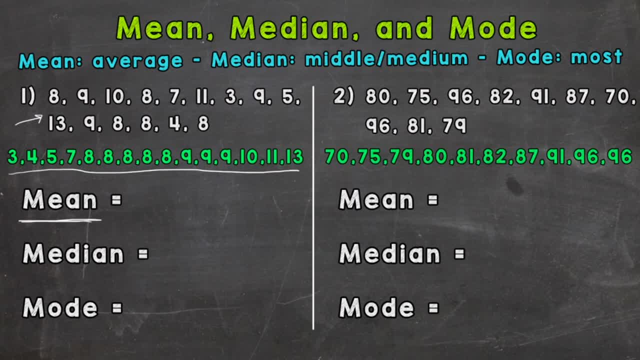 So for this, this group of numbers, when we add them up, the sum is 120.. Now there are 15 numbers in this set. So we would do 120 divided by 15. And that would give us an average or mean of eight. 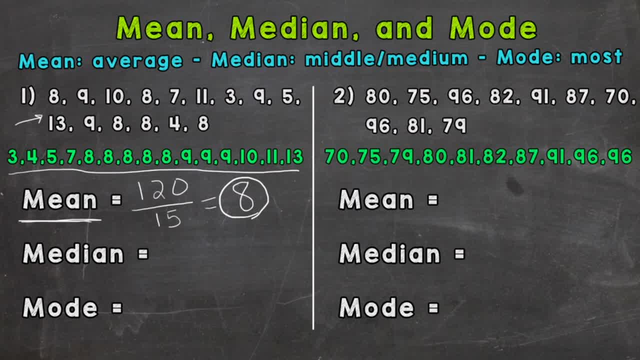 So again, mean is the typical average we think of, And that's when we add up all the numbers And then divide by how many numbers there are in that set. Now, median, you can think medium or middle, It's the middle number. once you list those numbers from least to greatest, 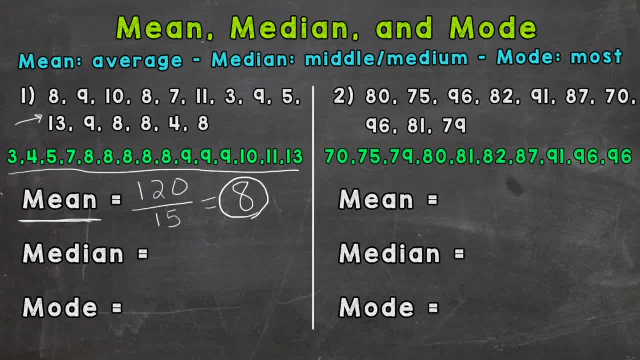 So there are 15 numbers in this list, So we should have seven numbers on each side of that middle number. So one, two, three, four, five, six, seven. one, two, three, four, five, six, seven. 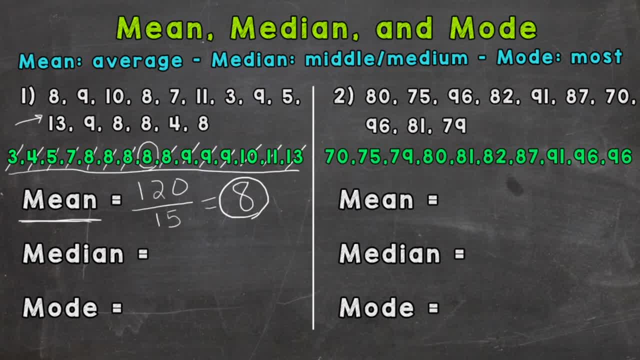 So one of the eight is sitting right in the middle. So that would be our middle medium, or the correct term would be median. So our median is eight as well. Now the mean and median are the same For number one. that's not always the case. 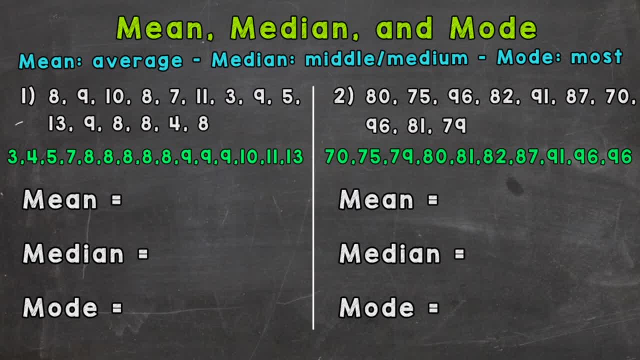 So for number one, we have a list of numbers up here. This is our data set Now below it in green: this list I already put in from least to greatest. So I put those numbers from least to greatest to help organize them. 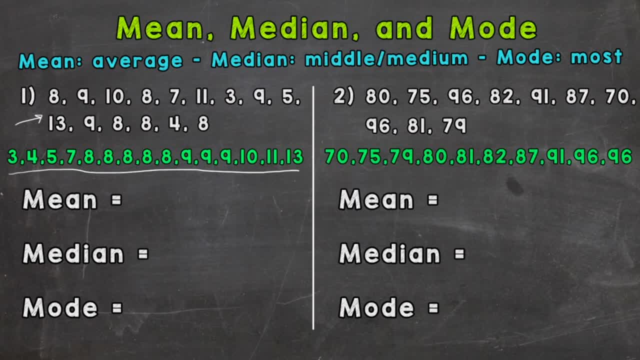 So whenever you have a list of numbers, order them from least to greatest first. Then we can find the mean, median and mode. So let's do mean first. And the mean is the typical average we think of when we add up all the numbers in the data set and then divide by how many numbers there are in that set. 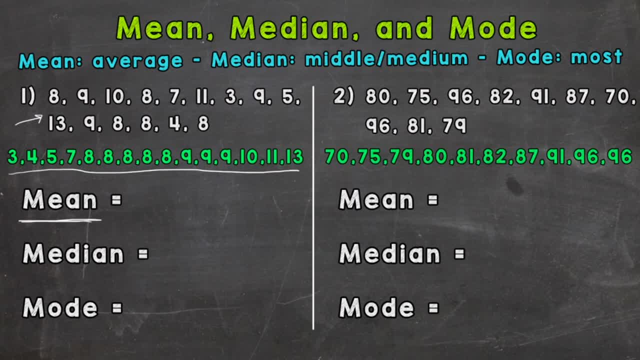 So for this, this group of numbers, when we add them up, the sum is 120.. Now there are 15 numbers in this set. So we would do 120 divided by 15. And that would give us an average or mean of eight. 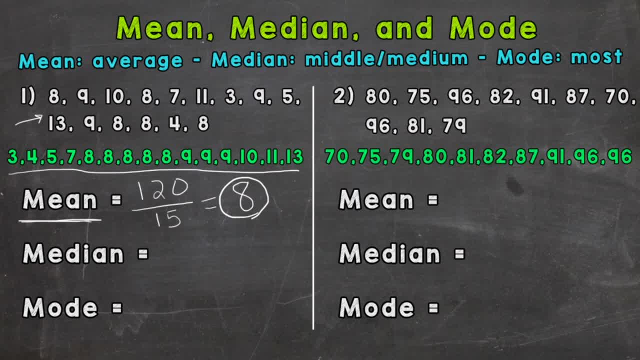 So again, mean is the typical average we think of And that's when we add up all the numbers. So we add up all the numbers and then divide by how many numbers there are in that set. Now median, you can think medium or middle. 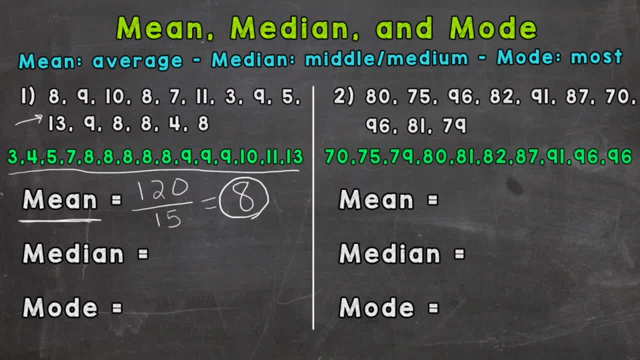 It's the middle number once you list those numbers from least to greatest. So there are 15 numbers in this list, So we should have seven numbers on each side of that middle number. So one, two, three, four, five, six. 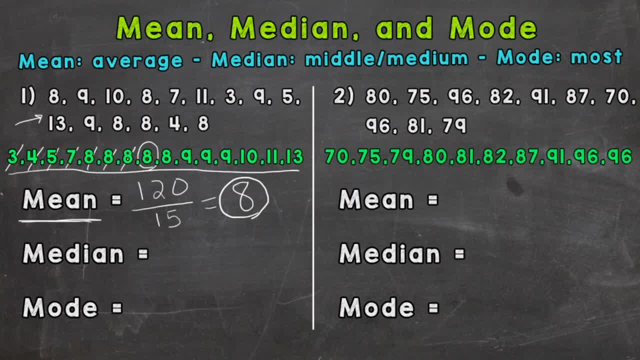 Seven. one, two, three, four, five, six, seven. So one of the eight is sitting right in the middle. So that would be our middle medium, or the correct term would be median. So our median is eight as well. 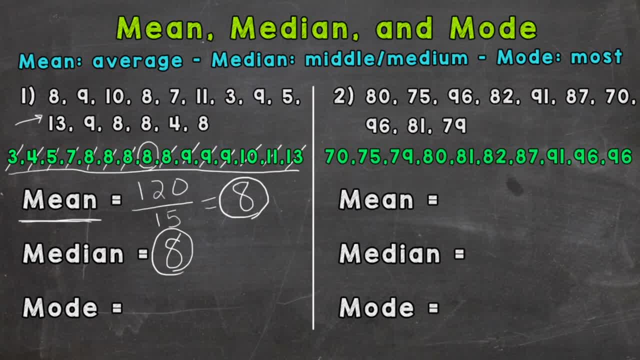 Now the mean and median are the same for number one. That's not always the case. They do not have to be. They're the exact same. Now mode you think most. What number occurs the most in that data set? So let's take a look here. 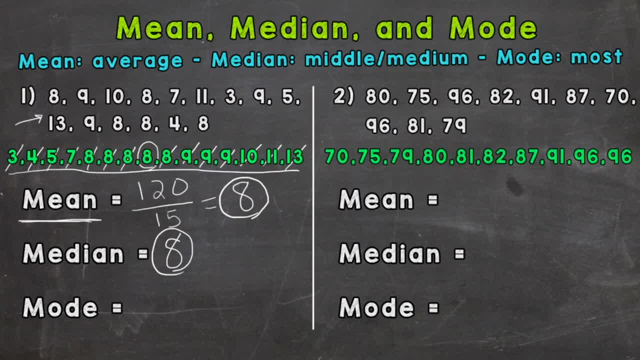 They do not have to be the exact same Now mode, you think most. What number occurs the most in that data set? So let's take a look here Now. three, four, five and seven all occur once. Then we have this group of eights. 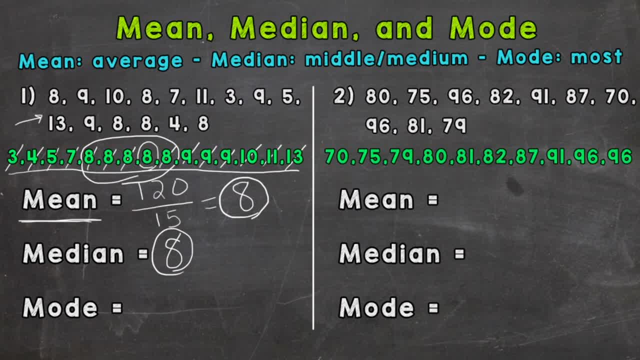 And we have five eights there. So let's double check if anything occurs more. We have three nines and then one 10,, one 11, and one 13.. So the number that occurs the most would be eight. So our mean median and mode are all eight. 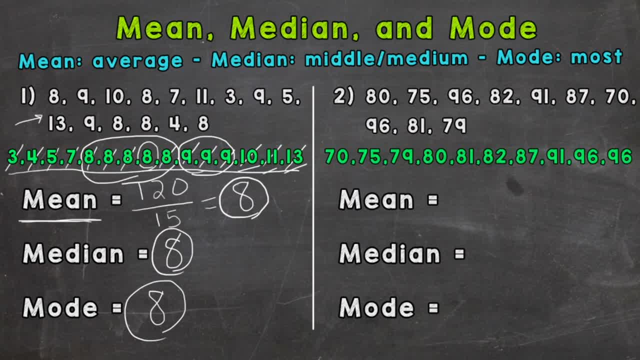 And, like I just explained, with the median they don't all have to be the same number And most of the time they won't end up being all the same number. So let's take a look at number two And we'll start with the mean. 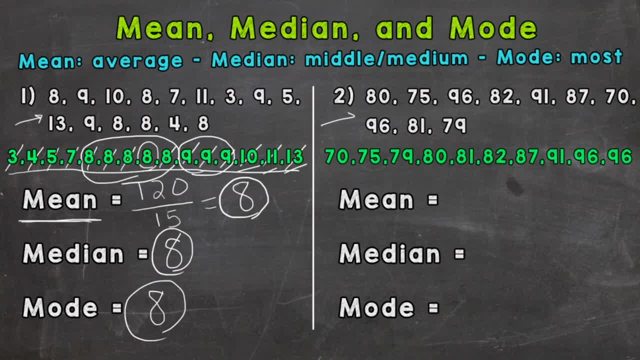 So again, the white numbers. right here is all the data mixed up. The green numbers below I took and listed those from least to greatest. So I organized everything, So let's do the mean first. So we need to add up all of the numbers. 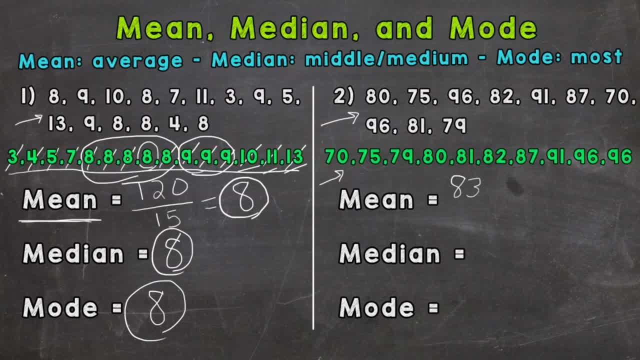 And we would get 837.. And we need to divide by how many, And we need to divide by how many, And we need to divide by how many numbers are in that list or data set, And we have 10.. So we would do 837 divided by 10 to find the mean or the typical average. 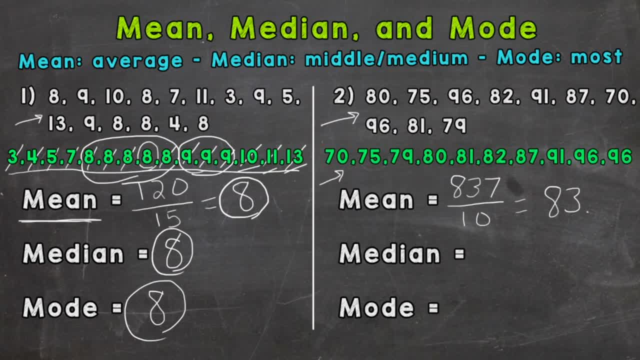 And we would get 83 and 7 tenths. So that would be our mean, Now median. we need to find the middle number And you can think medium or middle. So we have 10 numbers in the data set. So that means we're going to have four numbers on each side here. 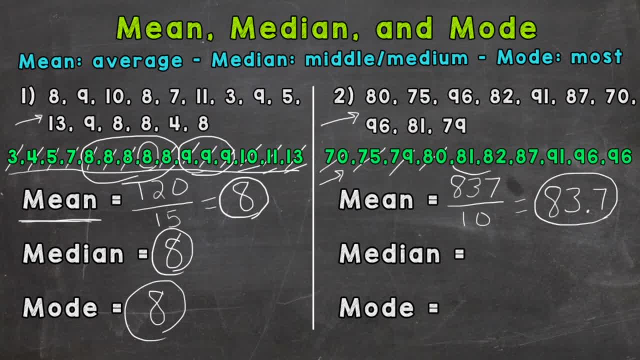 One two, three, four, One two, three, four And we actually have two numbers in the middle. So if that happens, you just take whatever is in the middle of those two numbers, So you can either add those two numbers 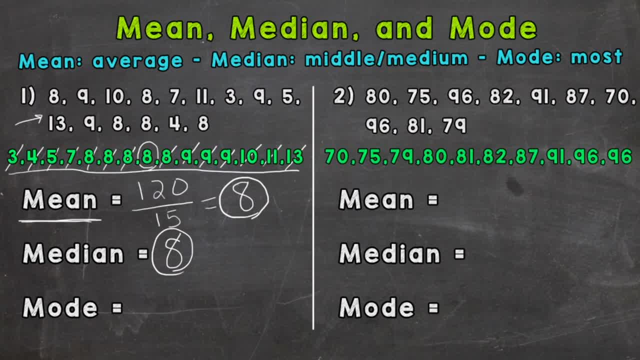 Now three, four, five and seven all occur once. Then we have this group of eights And we have five eights there. So let's double check if anything occurs more. We have three nines And then one ten, one eleven. 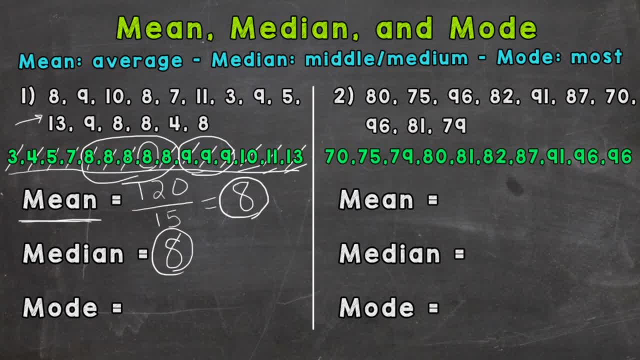 And one thirteen. So the number that occurs the most would be eight. So our mean median and mode are all eight And, like I just explained, with the median they don't all have to be the same number And most of the time they won't end up being all the same number. 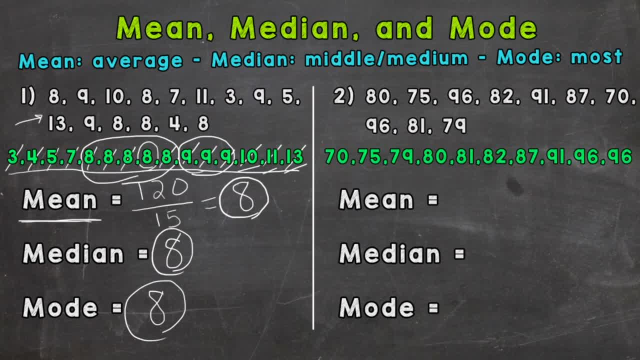 So let's take a look at number two And we'll start with the mean. So again, the white numbers. right here Is all the data mixed up. The green numbers below: I took and listed those from least to greatest, So I organized everything. 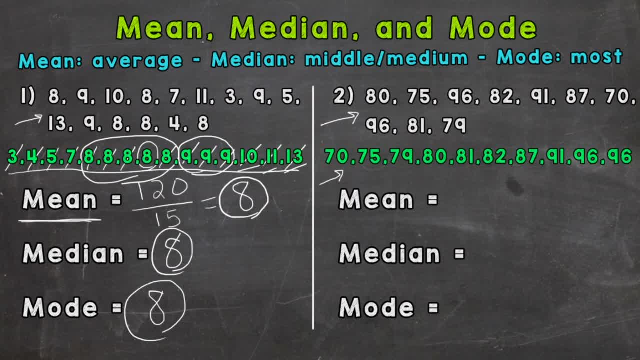 So let's do the mean first. So we need to add up all of the numbers And we would get eight hundred thirty-seven And we need to divide by how many numbers are in that list or data set And we have ten. So we would do eight hundred thirty-seven divided by ten to find the mean or the typical average. 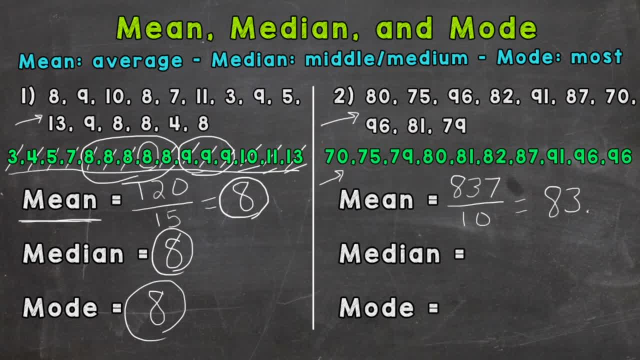 And we would get eighty-three and seven tenths. So that would be our mean, Now median. we need to find the middle number And you can think medium or middle. So we have ten numbers in the data set. So that means we're going to have ten numbers in the data set. 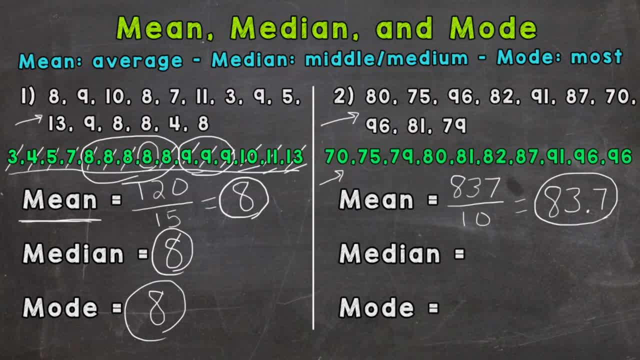 So that means we're going to have four numbers on each side here, One two, three, four. One two, three, four, And we actually have two numbers in the middle. So if that happens, you just take whatever is in the middle of those two numbers. 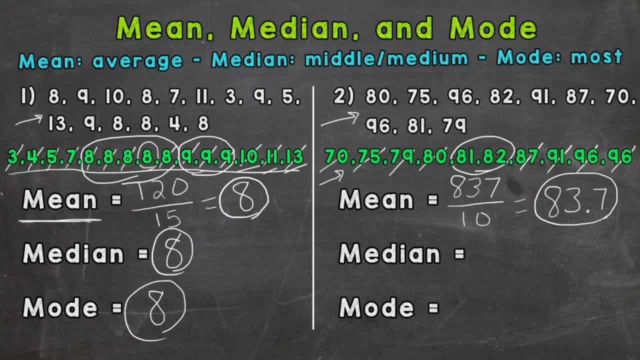 So you can either add those two numbers up and divide by two, And that will give you exactly what's in the middle, Or for this we look at eighty-one and eighty-two and we know that eighty-one and a half is right in between eighty-one and eighty-two. 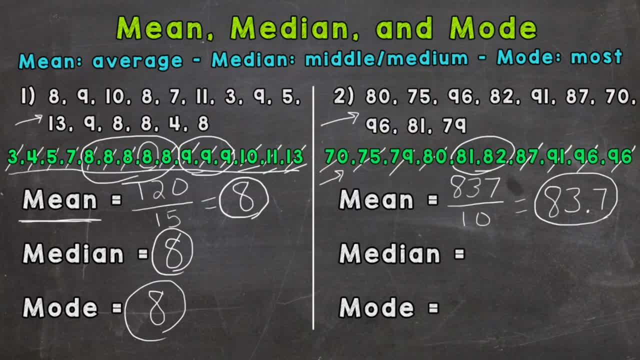 You can either add those two numbers up and divide by two, And that will give you exactly what's in the middle of those two numbers, Or for this we look at 81 and 82. And we know that 81 and a half is right in between 81 and 82.. 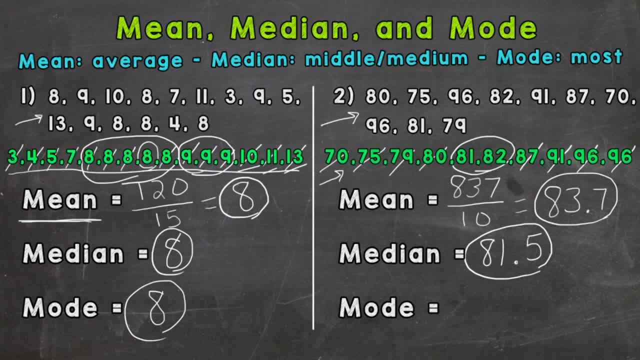 So our median would be 81 and 5 tenths. And we'll end with mode, And remember mode means most, So what number occurs the most In that data set? So 170, 175, 79, 80,, 81,, 82,, 87, 91. 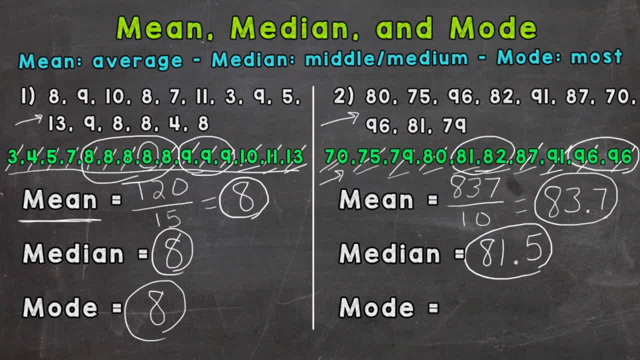 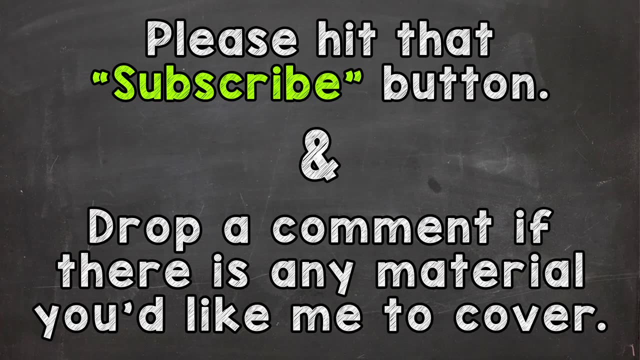 And we have two 96s, So that 96 would be our mode the most occurring. So there you have it: Mean median and mode. Thanks so much for watching, Until next time, peace. 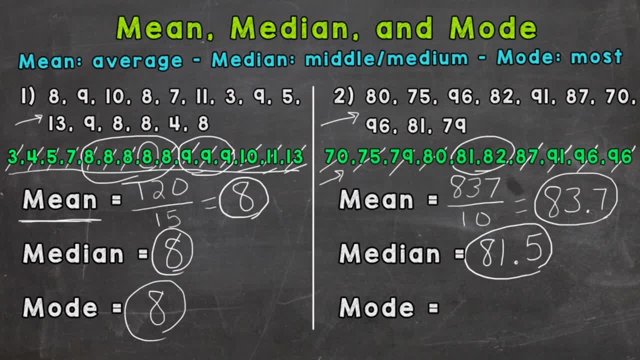 So our median would be eighty-one and five tenths. And we'll end with mode, And remember, mode means most, So what number occurs the most in that data set? So one-seventy, one-seventy-five, seventy-nine, eighty, eighty-one, eighty-two, eighty-seven, ninety-one, and we have two ninety-sixes, so that ninety-six would be our mode the most occurring. 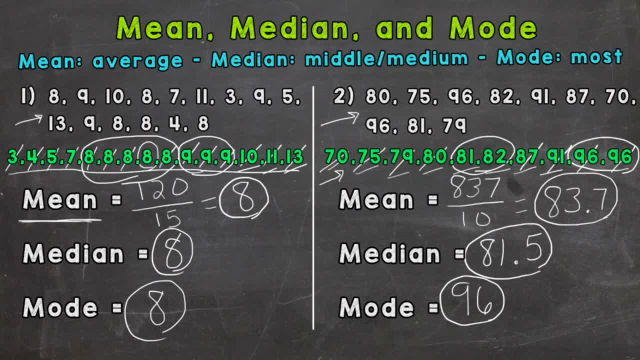 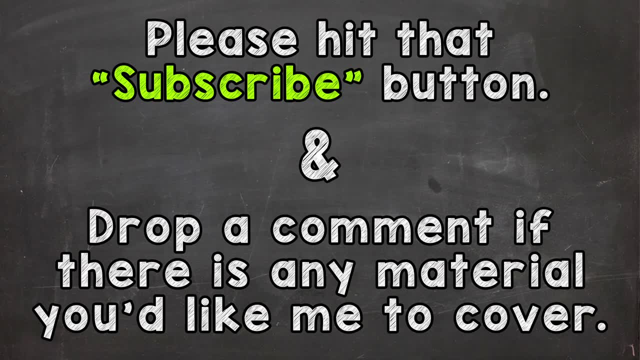 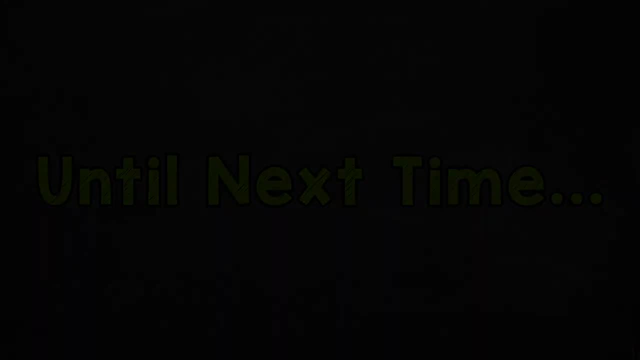 So there you have it: Mean, median and mode. Thanks so much for watching. Until next time, peace. Thanks for watching. 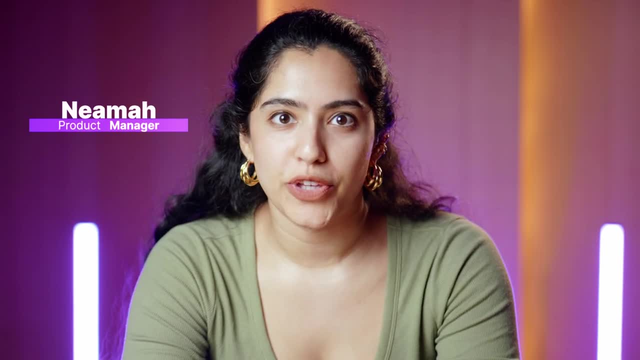 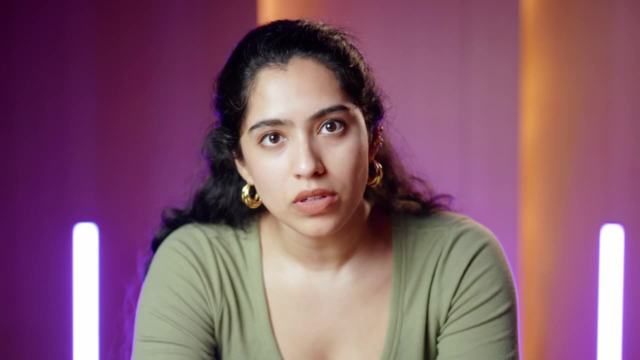 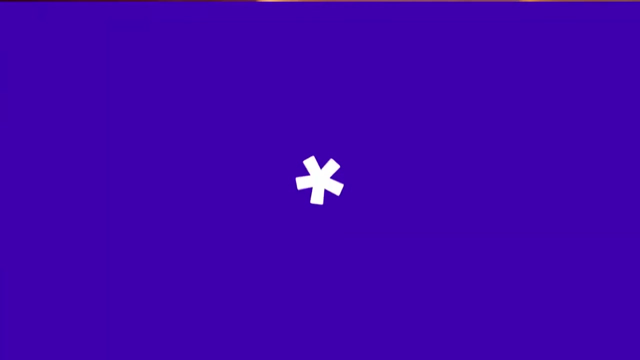 Let's talk about how to choose a database in a system design interview. In these interviews, you will often have to choose what database to use, and these databases are split into SQL and NoSQL types, and they each have their own strengths and weaknesses and should be chosen appropriately based on the use case. First, let's define both SQL and NoSQL databases. 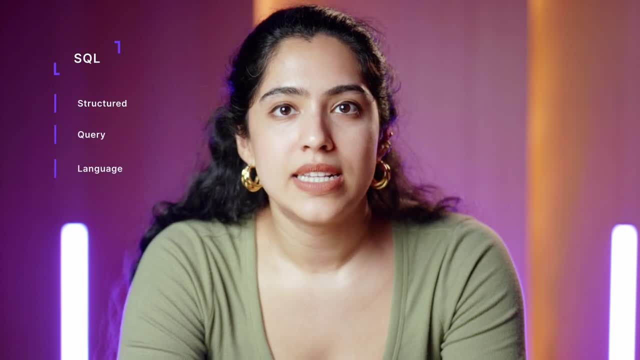 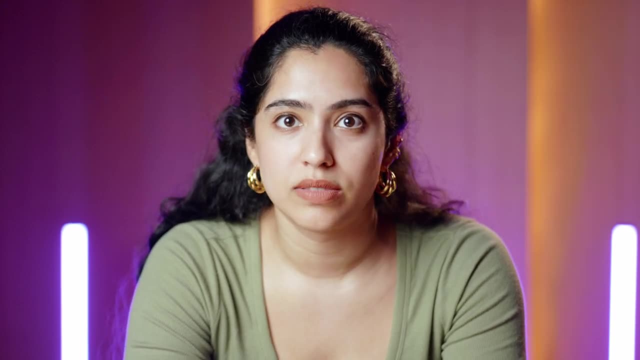 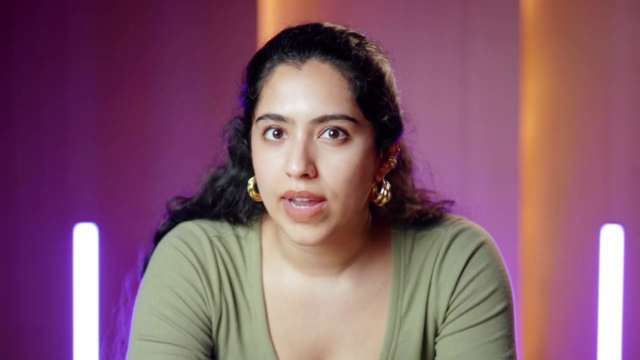 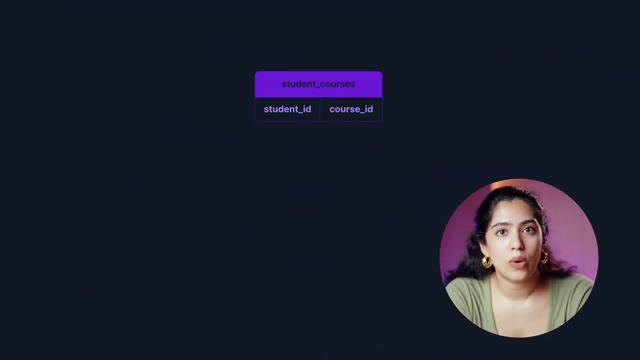 SQL stands for structured query language. SQL databases are table based, while NoSQL are document, key, value, graph or wide column stores. SQL databases are vertically scalable, while NoSQL databases are horizontally scalable. Let's start with the strengths of SQL databases First. SQL databases are relational databases, which means that they allow easy querying on.